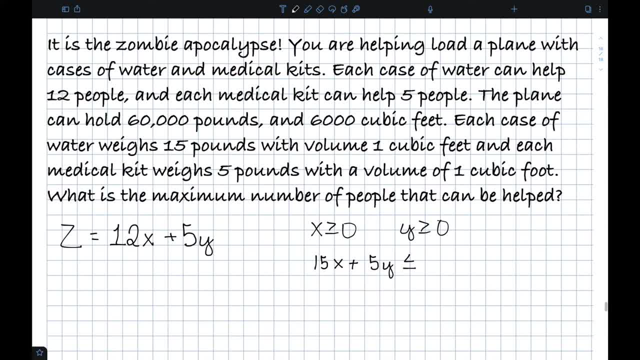 Medical kits weigh 5 pounds, And that has to be less than or equal to 5 pounds, And that has to be equal to my maximum weight, 60,000.. I also have to be concerned with volume. Water and medical kits are both 1 cubic foot, so x plus y. 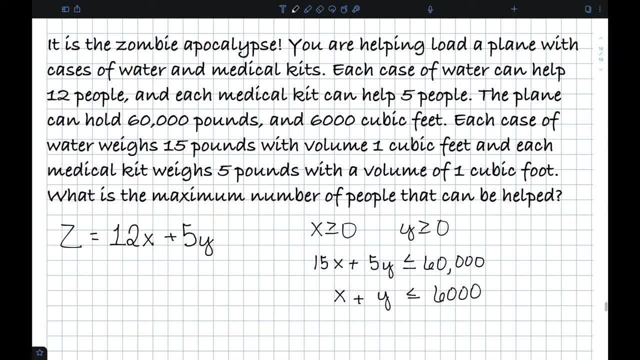 And that has to stay less than 6,000.. So now that I have my constraints, let's solve this system. Let's start by graphing the inequalities: The x greater than or equal to 0, and y greater than or equal to 0.. 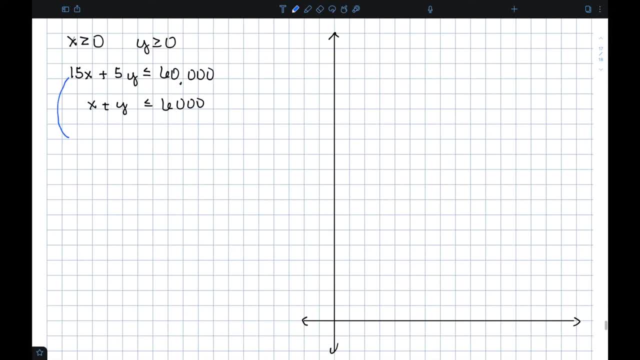 Just tells me I'm in this first quadrant. And let's look at the intercepts. My first equation: if I let x be equal to 0,, I have 5y equal to 60,000.. Or y is equal to 12,000.. 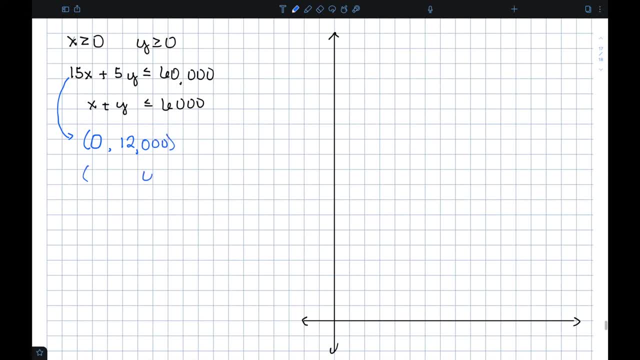 If I let y be equal to 0,, I have 15x equal to 60,000.. Dividing both sides by 15 gives me 4,000.. So as I graph this, I'm going to let each one of these boxes be 1,000.. 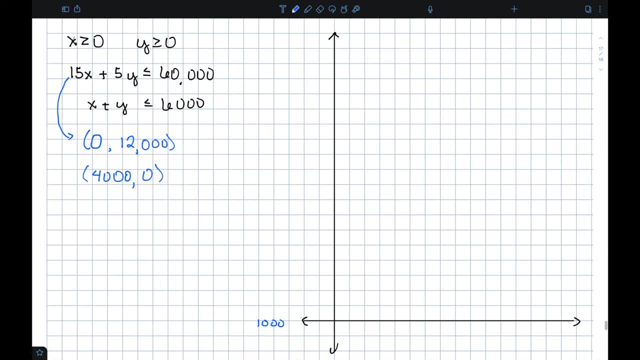 I should be able to go over 0, and up 1,, 2,, 3,, 4,, 5,, 6,, 7,, 8,, 9,, 10,, 11,, 12.. I should also be able to go over 4,, 1,, 2,, 3,, 4, and up 0. 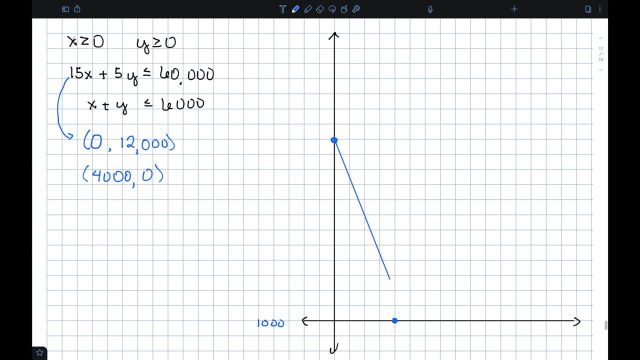 And we can connect these dots. Since 0 plus 0 is in fact less than 60,000,, I should be shading on the side of the line that has 0, 0.. Next, if x is 0, we can see that y has to be 6,000.. 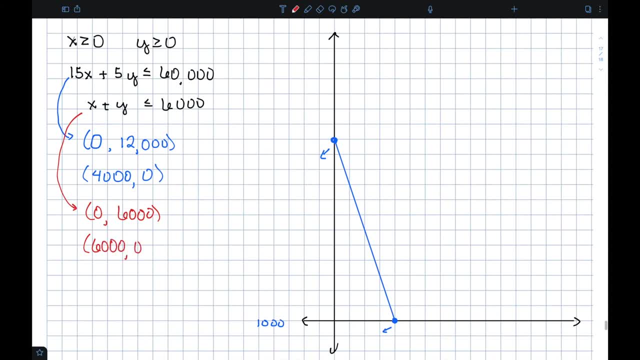 And if y is 0, we can see that x has to be 6,000.. So I can plot Those two points- 6,000, 0, and 0, 6,000, and connect the line between them. 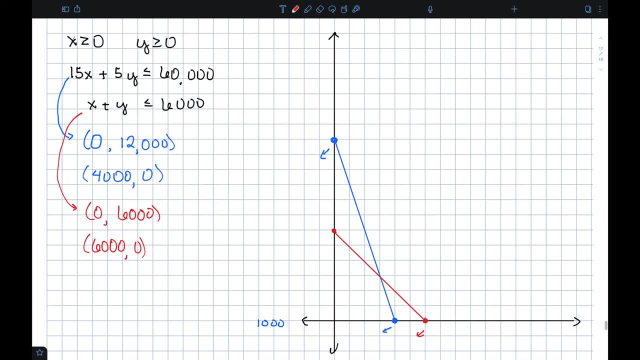 And once again, since 0 plus 0 is in fact less than 6,000, I need to shade below this line, So I need to be below the red and below the blue and positive, Finding my vertices. I already know this one is 0, 6,000.. 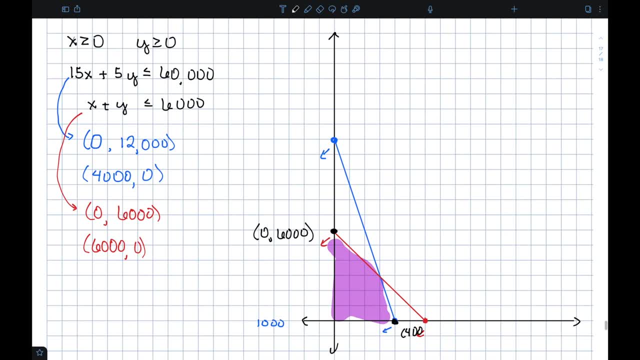 And I already know this one is 4,000, 0.. And I also have the point 0, 0.. I just need to figure out where this is. Where do these two lines intersect? Where is 15x plus 5y equal to 60,000?? 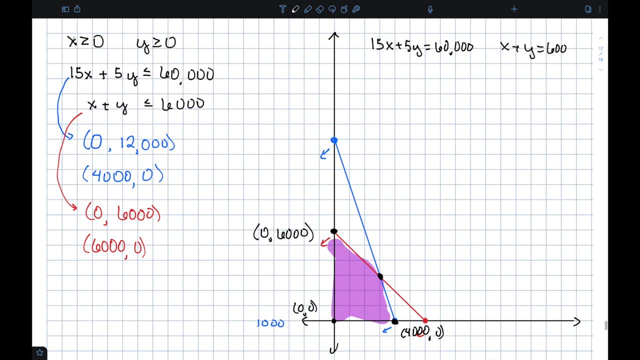 And x plus y equal to 6,000. the same. Well, I'm going to multiply this second one by minus 5.. That gives me negative 5x minus 5y equal to negative 30,000.. That tells me 10x is equal to 30,000.. 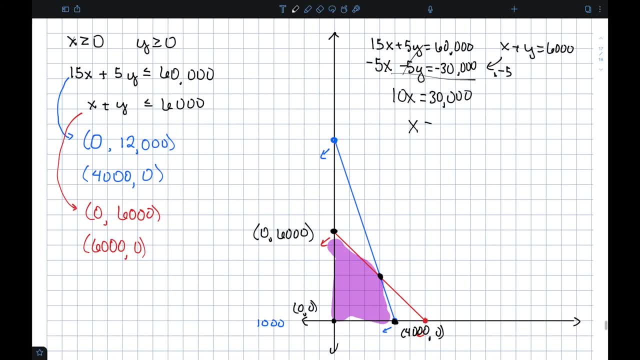 Or if I divide both sides by 10, x is equal to 3,000.. Solving for y, I'm going to use the fact that x plus y has to be equal to 6,000. to get that, y must also be 3,000.. 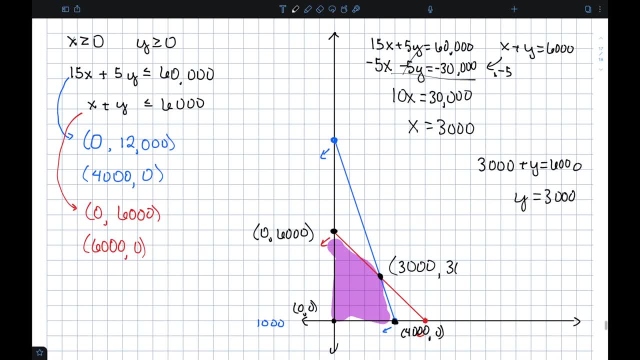 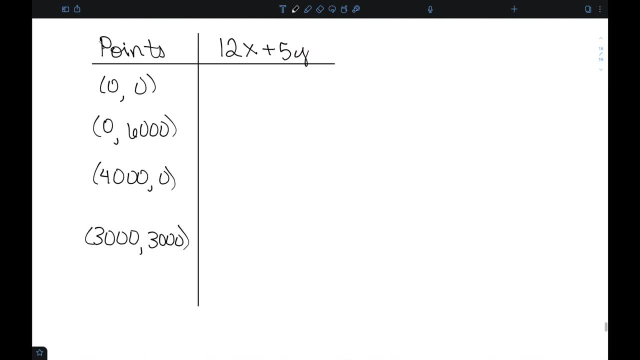 So this is the point: 3,000, 3,000.. We can now plug these points into my objective function. If we send 0 medical kits and 0 bottles of water, we will of course, help 0 people. The next one, 12 times 0, is 0.. 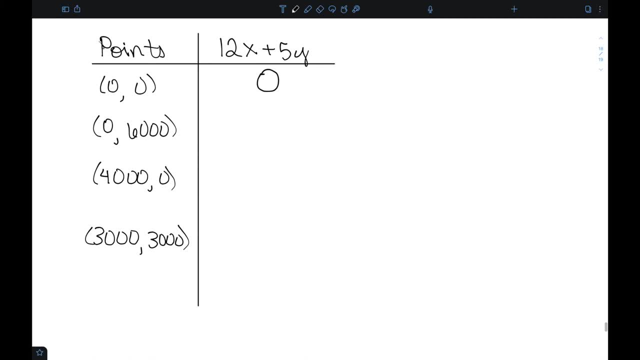 And 5 times 6,000 is 30,000.. So this one would help 30,000 if we packed only medical kits. 12 times 4,000 is 48,000.. And then 5 times 0 is 0.. 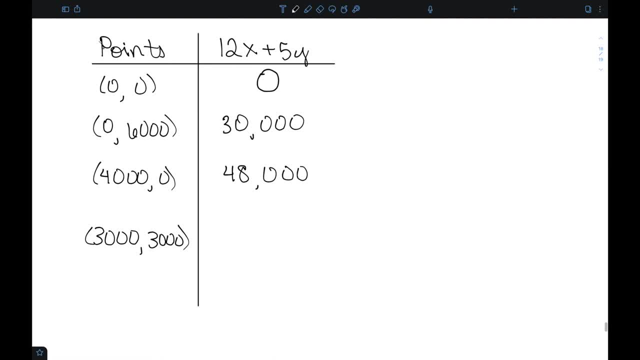 So if we packed only water, we could help 48,000 people. 12 times 3,000 is 36,000.. And 5 times 3,000 is 15,000.. So together, if I add those, I would get 51,000..